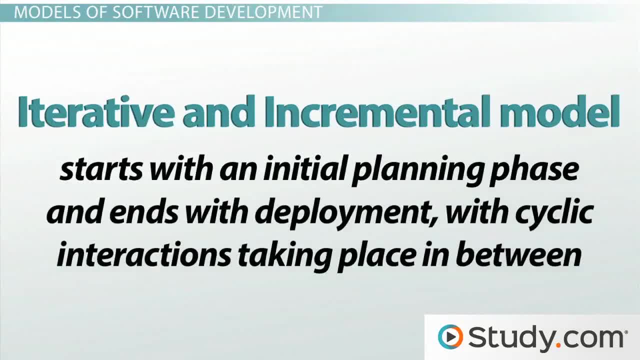 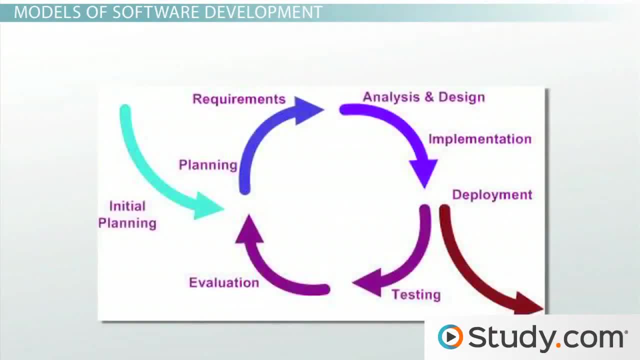 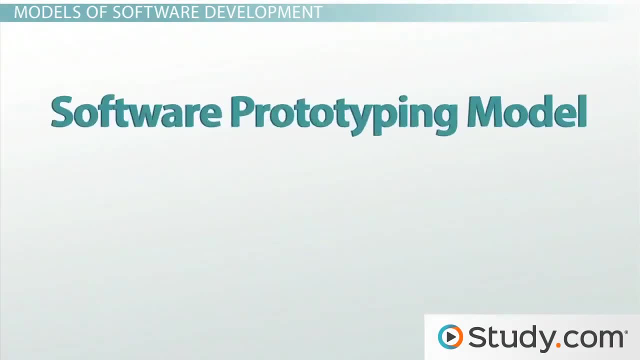 It starts with an initial planning phase and ends with deployment, with cyclical interactions taking place in between. The approach is incremental, since it divides the functionality into small increments which are developed and tested over one or more iterations. The software prototyping model relies on creating and testing prototypes of software applications. 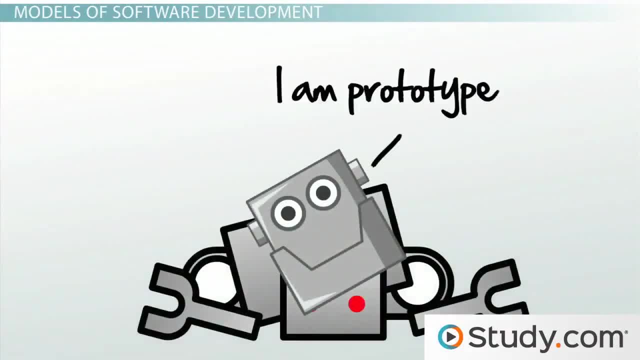 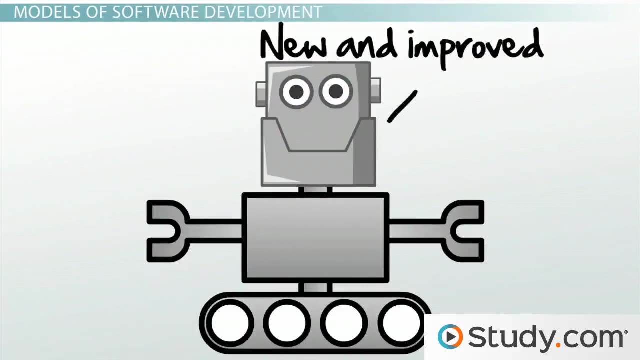 A prototype is a simple, incomplete version of the software being developed. An initial prototype is developed that meets some of the very basic requirements but lacks many of the details. The trial is a short and easy process. The initial prototype is tested and reviewed, and the feedback is used to improve the prototype. The spiral model.